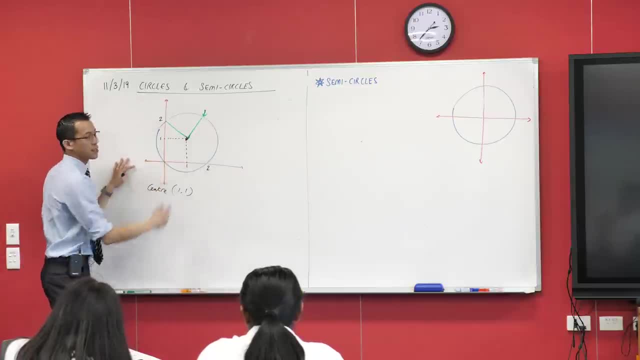 Okay, so I could go up to here, right From the centre to this spot on the circumference that will be the radius. go ahead and say there's an even easier place you could go. the origin is also right on the circumference right, and because that's there I can draw myself. 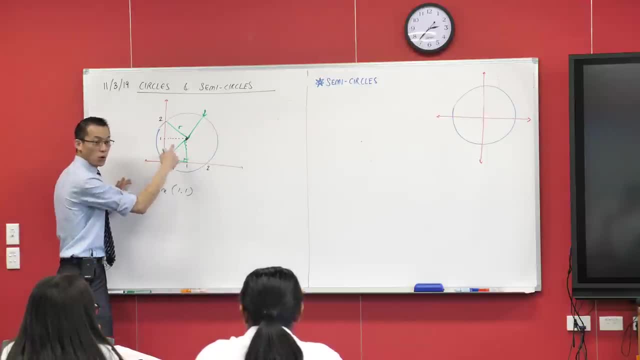 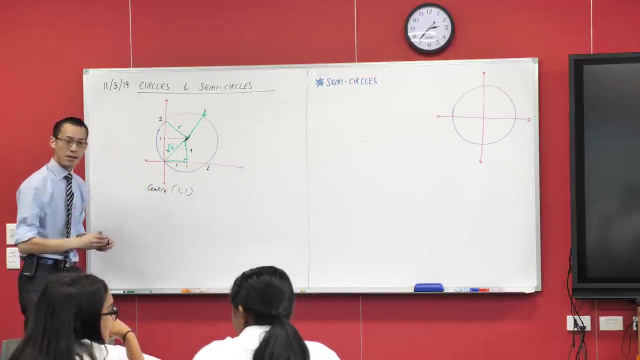 a nice neat right angle triangle and you already know how tall the right angle triangle is. it's one. you know how wide the right angle triangles is, also one. so you can use what we started off today with Pythagoras and you're okay. oh, this is 1, 1 and root 2. so if that's the radius, if the radius equals root 2, what? 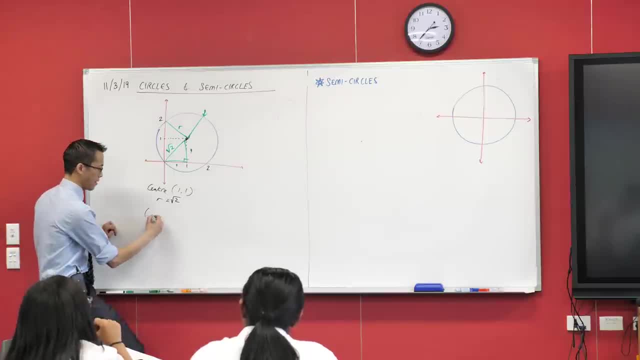 will the equation be? let's start with some brackets rather than throwing out random numbers. okay, hey, Sean, do you want to start us off? don't do the whole thing, just start us off, okay, so I'm gonna have something square. it's gonna be X minus 1 or square. can someone else take a? 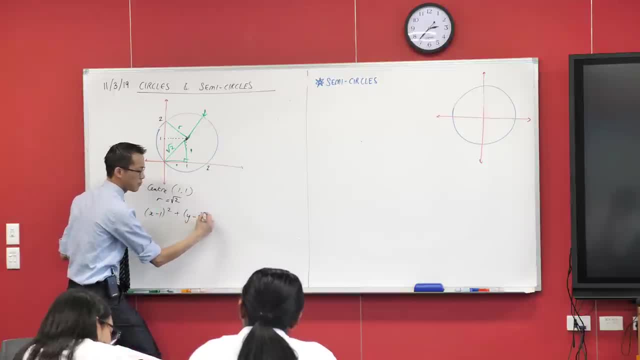 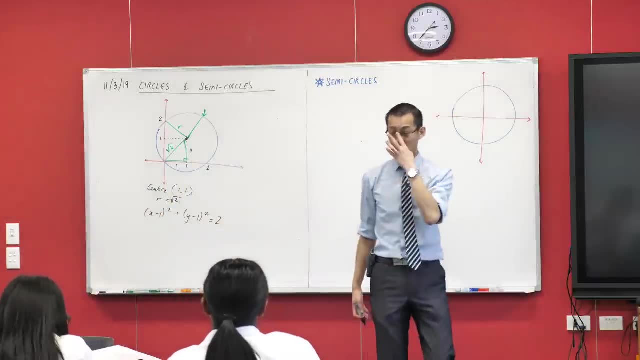 I've done the X, so I'm gonna do Y minus 1 or square, and then that equals to just 2, because the square root of the right hand side, in my nicely form, that's it. that's the radius to understand semicircles before we get to all these. 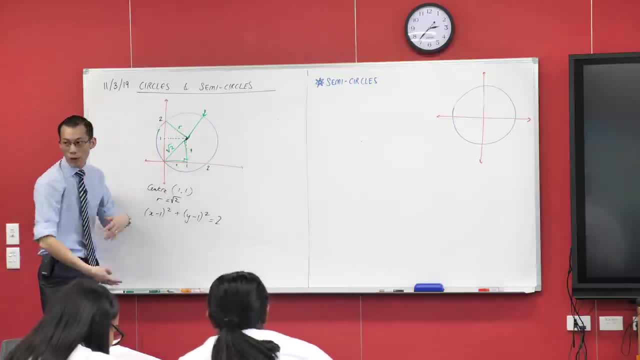 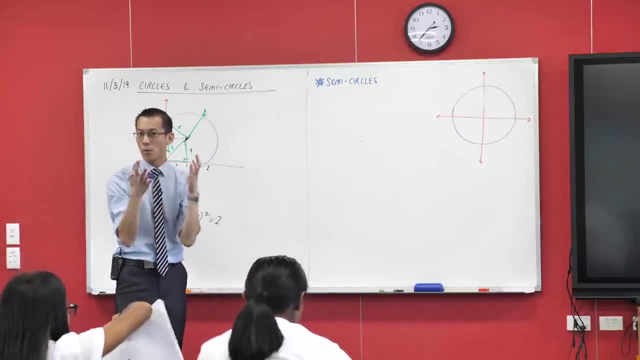 weird, wacky, crazy ones with weird centers and weird radii. it's often helpful in maths to, when you're going into a new area, start with the simplest version of what you can. now, what was the simple object that we started today with? we didn't just look at any circle, we look 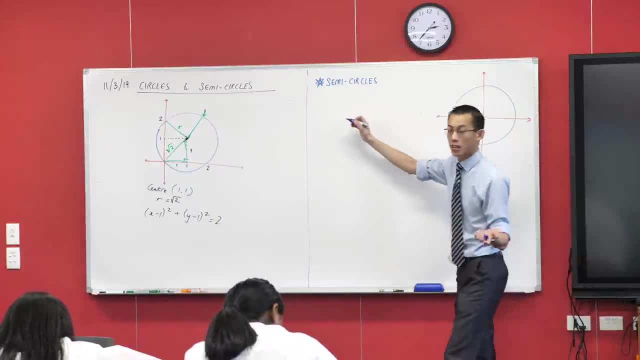 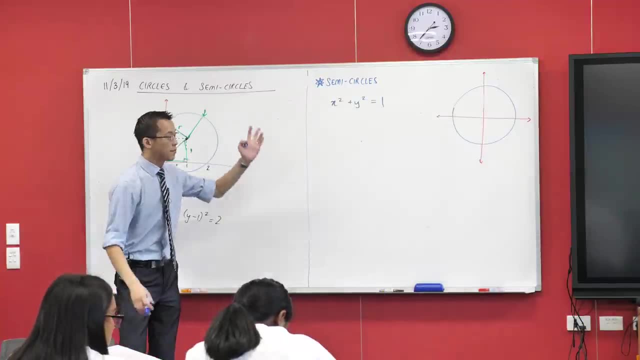 at a specific one, the unit circle, right? so we're going to start with the unit circle again, right? this guy here. x squared plus y squared equals 1. it's a nice simple object and we can use it- bless you- to work out what semicircles. 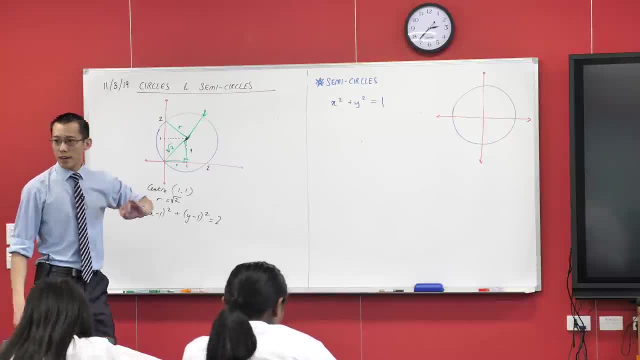 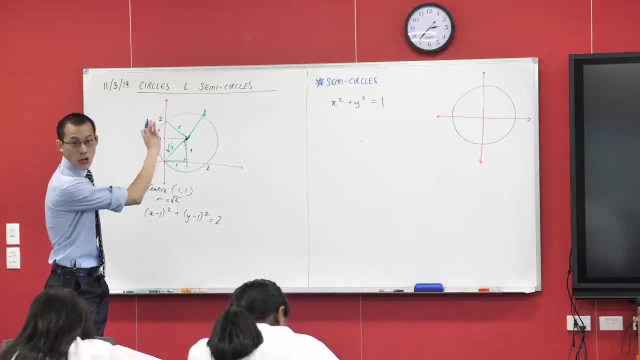 are like: okay, now x squared plus y squared centers at the origin radius is equal to 1. what I'm going to do here with you is if we make, if we rearrange this equation such that we have X or Y as the subject, it will make it really easy to see what. 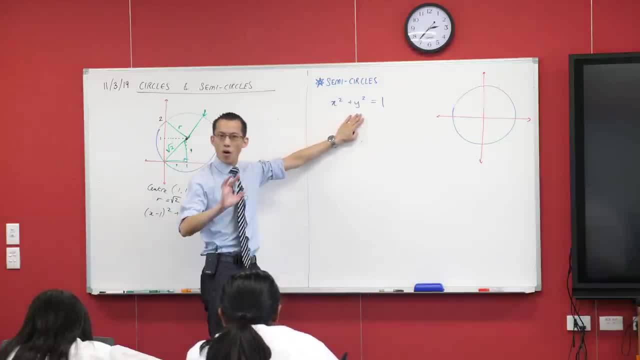 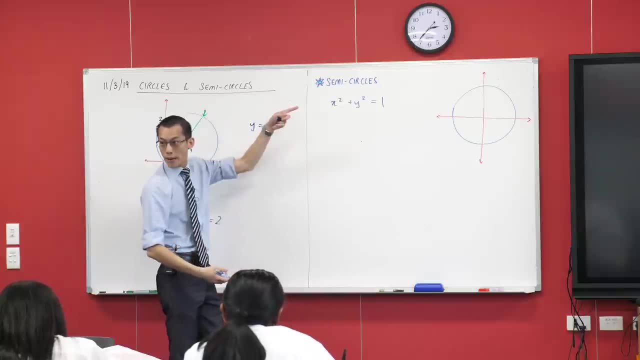 the semicircle is. let me show you okay, for instance, all of the parabolas and hyperbolas and straight lines. we're used to seeing them in this form: right: y equals whatever, y equals MX plus C, or y equals ax squared plus B, X plus C or 1. 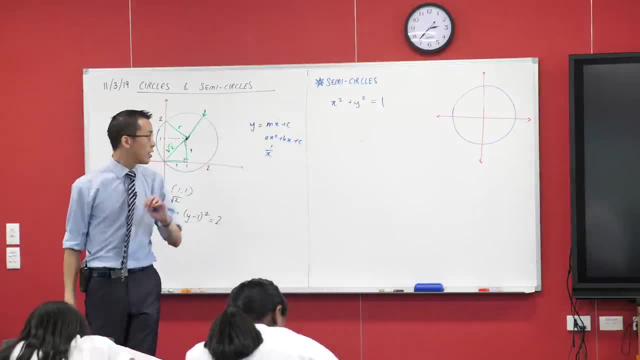 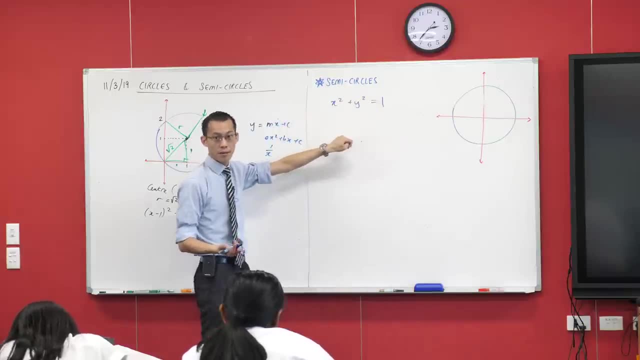 on X or whatever right. we usually make Y the subject, so here what would happen? what do I need to do first to make Y the subject? can anyone tell me the first step that might be helpful. okay, I'm going to subtract. see this: x squared is equal to 1 minus x squared. 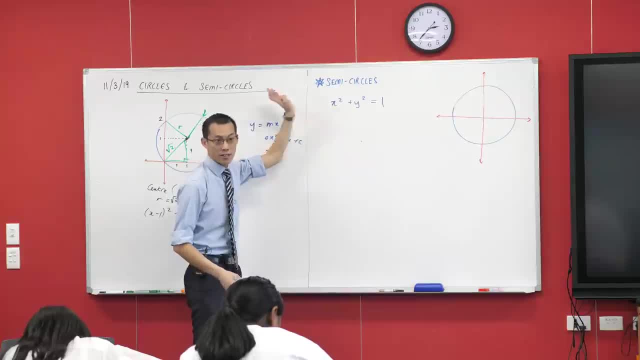 here, as Rasmus identified, that doesn't belong. I want it to be on the other side, so I'm going to subtract from both sides so you can follow along with me. I get this so far, so good. now, I wanted a y equals some stuff, right, not a y squared. 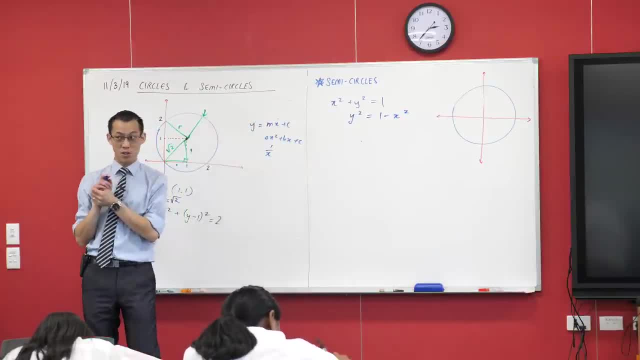 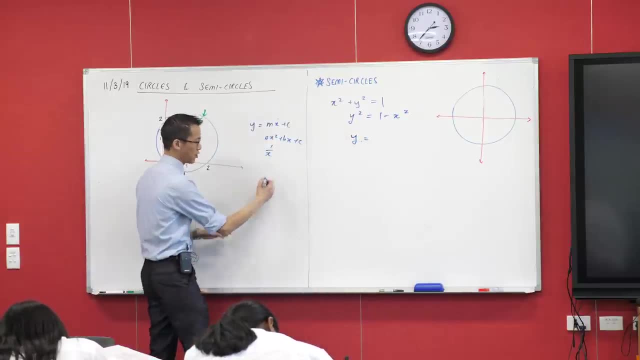 equals some stuff. so if I've got something squared, what should I do? both sides take the square root right now. just be cautious with this next bit, because if, for example, you had a question, you don't need to write this down. if I had a question like this: x squared equals 25, right? 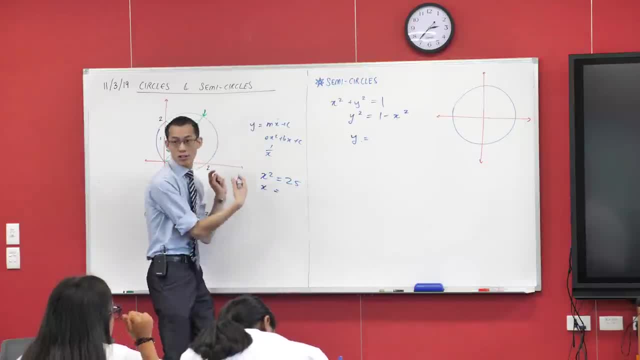 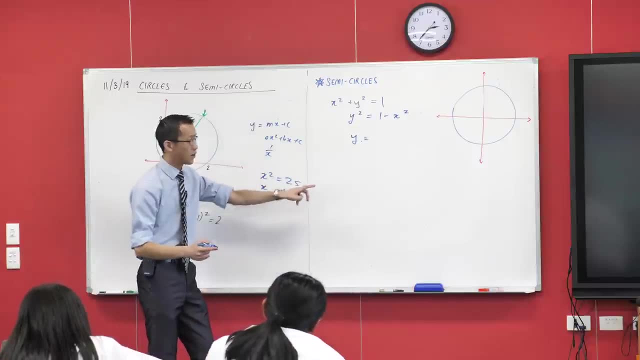 you can take the square root on the left hand side, but you know you don't just write a single number on the right hand side, right, it's not just 5, it's plus or minus, because both of those can get squared to give you 25- same thing. 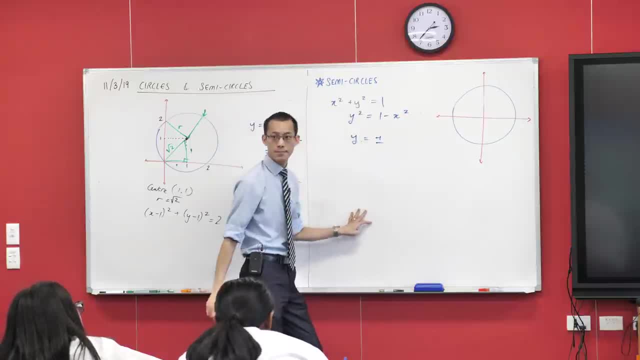 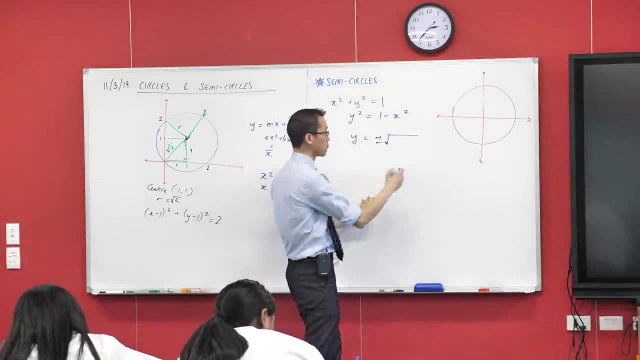 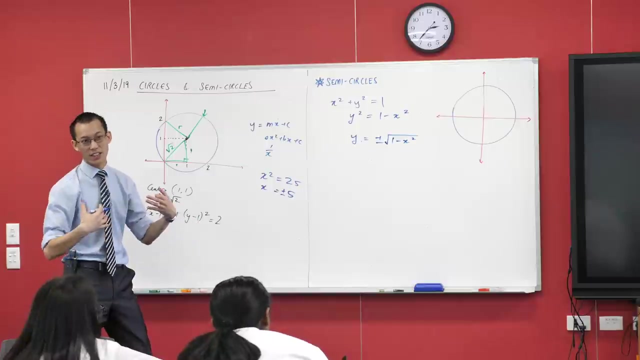 applies here. so I'm going to write plus or minus. and then what do I write? square root of all of the stuff that's here: 1 minus x squared. okay, now what this is. remember, plus or minus is just a lazy mathematicians way of saying two separate things, and I'd love us to write. 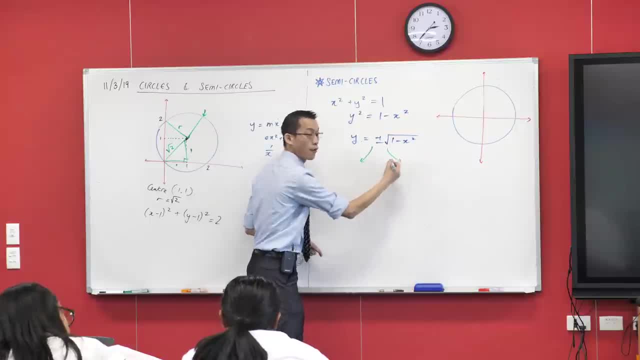 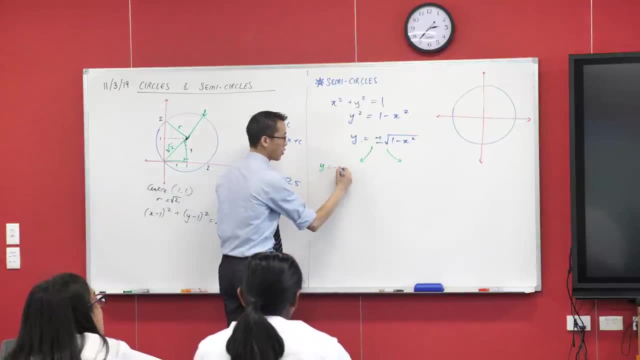 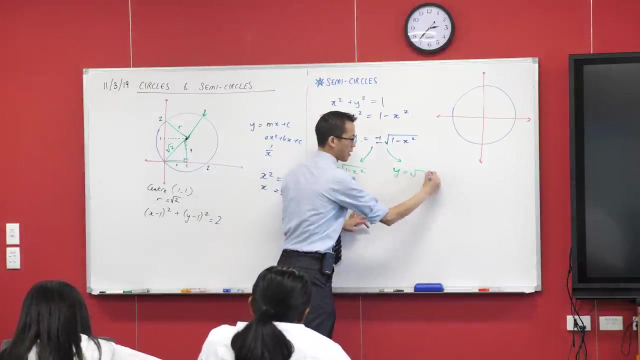 what those two separate things are. so this is shorthand for, just like in the quadratic equation to a quadratic formula, sorry, two completely separate things. there's the negative one, like this, and then there's also the positive one when there's a plus 1 minus x squared. okay, now what you're staring at. 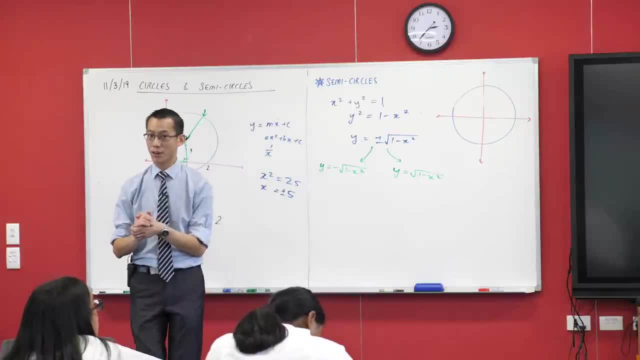 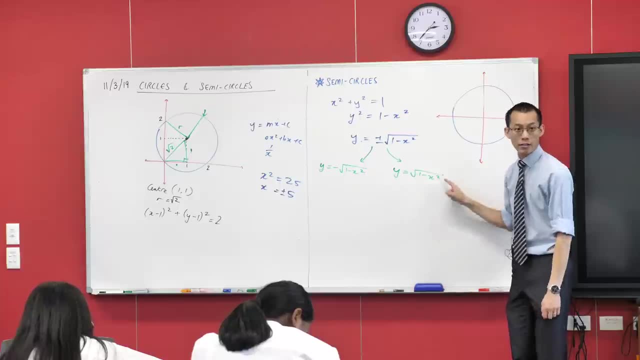 right now are two semicircles right and you can tell me which ones they are? because the square root- this guy over here, when it's positive, this thing is only, can only be positive values. right, like I know that this is plus or minus 5, but what's the square root of 16? 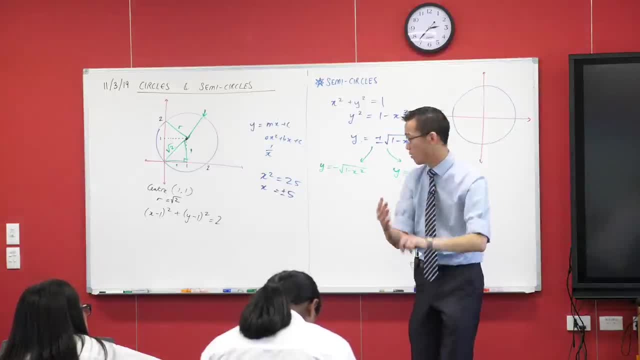 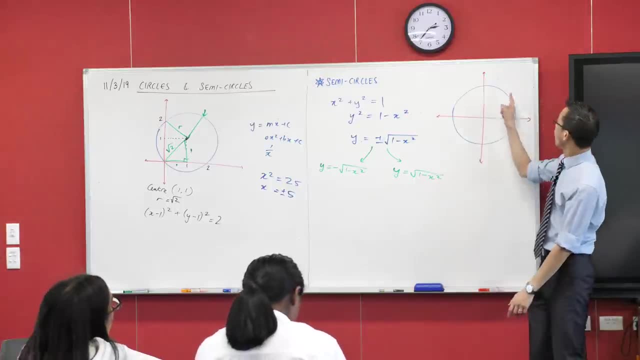 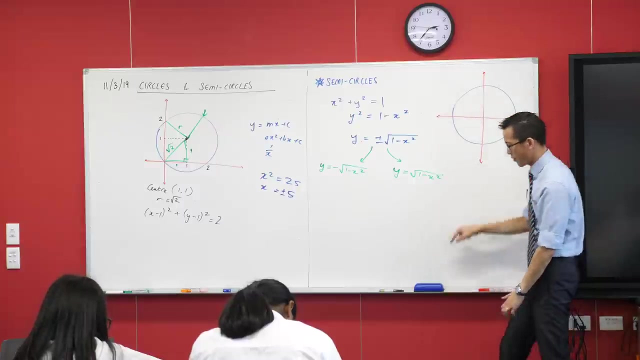 it's just 4. it's not negative. 4 right, it's just 4. so see this guy here. this is only positive, so the range of this is going to be above 0. so where on my unit circle will this be? it's going to be that the top part, right? so this guy up here, in fact. 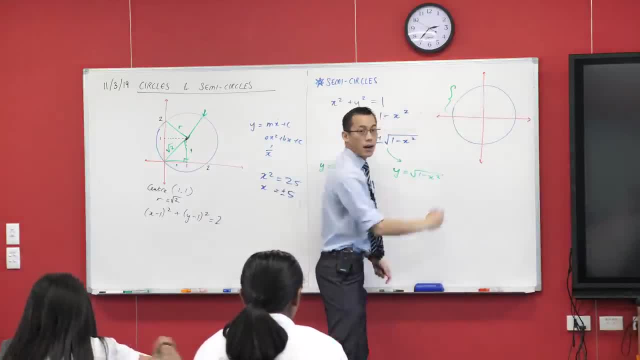 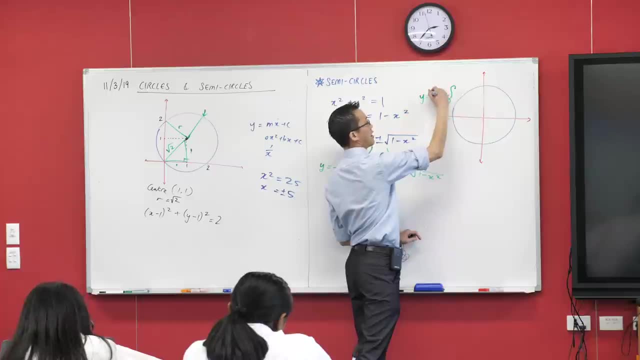 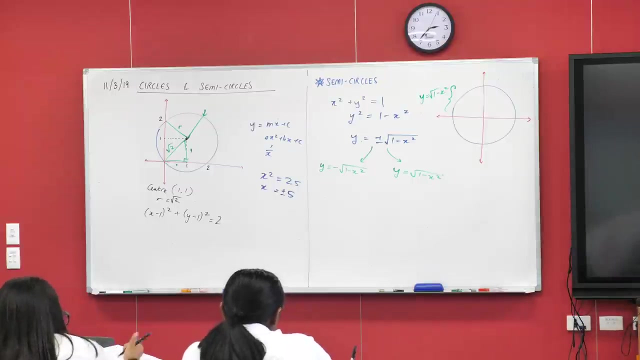 moving and draw it as such. this guy up here is the positive square root of 1 minus x squared. does that make sense? this is: y equals the square root of 1 minus x squared right. and you know, you might have Desmos nearby, you might be. 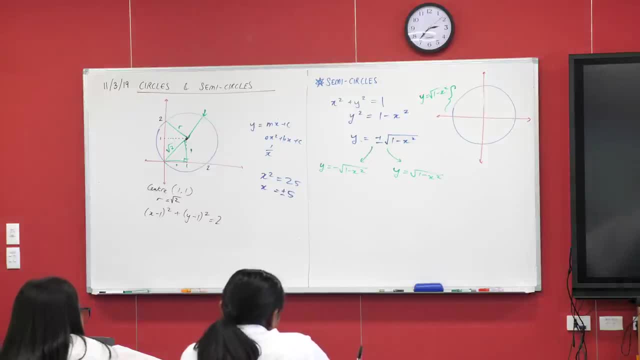 able to chuck in. y equals the square root of 1 minus x squared. there is right. so there's our semi circle, just like we expected. okay, what's the other part can tell you, because this is like both of them. this one says both of those if 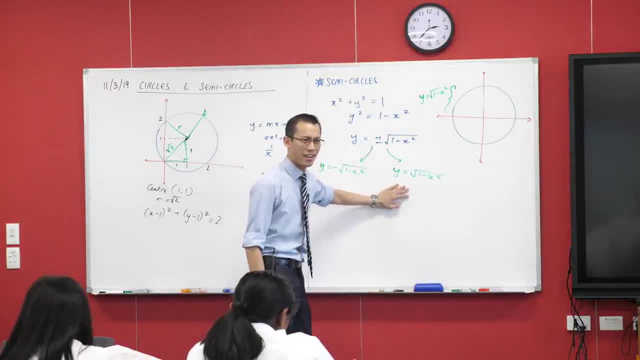 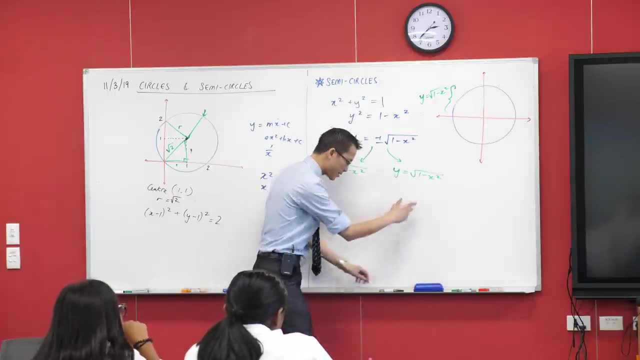 this is sorry, said yes, what's x squared? yes, so it kind of looks like a parabola right unit, X way, but that's square root kind of turns into the circle. so see how, this is the top half. right, this is the top half. what happens when you slap a? 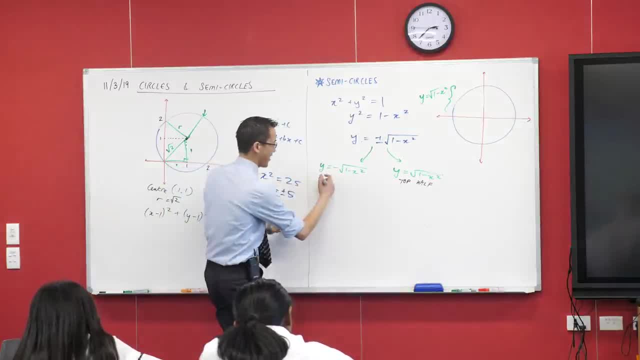 minus sign on the front, it gets 2 Square root. then here appears x squared. it's minus sine over here. times y gives you the bottom half right. So this is underneath. So if you go to Desmos and you just chuck a minus sign at the front, 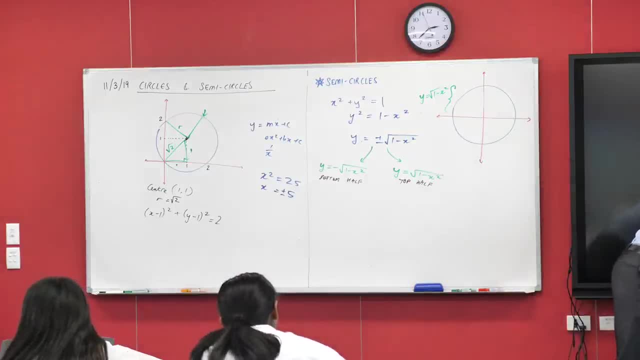 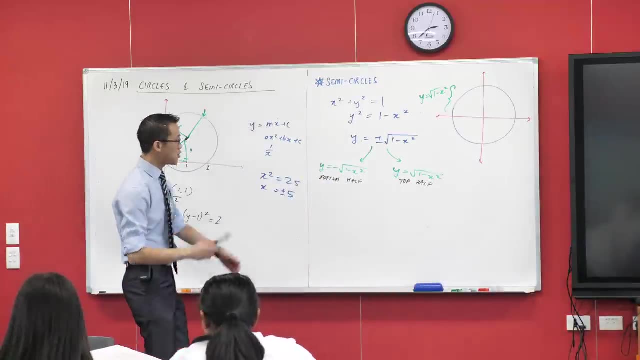 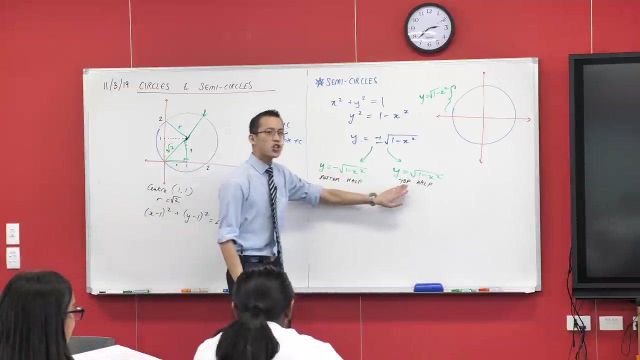 bam, There you go. There's the underneath, There's the other semicircle. okay, So you've got top half. it's the plus. You've got the bottom half. look at that minus sign. that's there. Okay, So this is top. 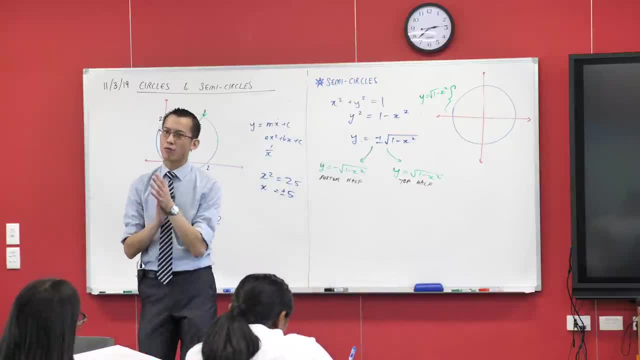 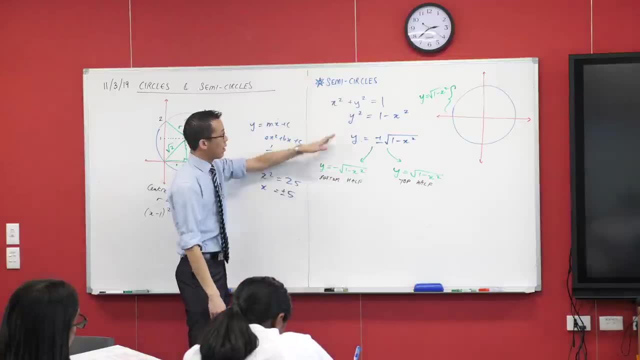 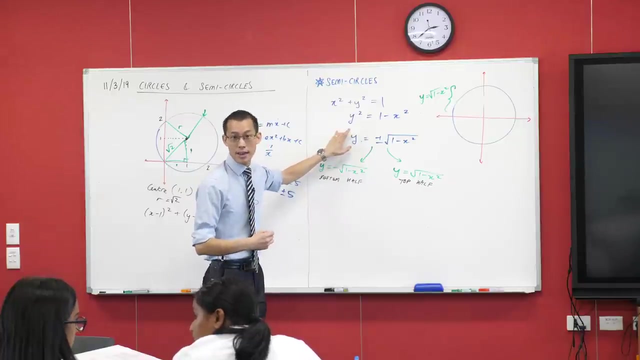 and bottom. How would we do left and right? What are you thinking? Ah, Okay, so you see how we went through, right? We started with this guy and we made y the subject. okay, If we went through and made x the subject instead? 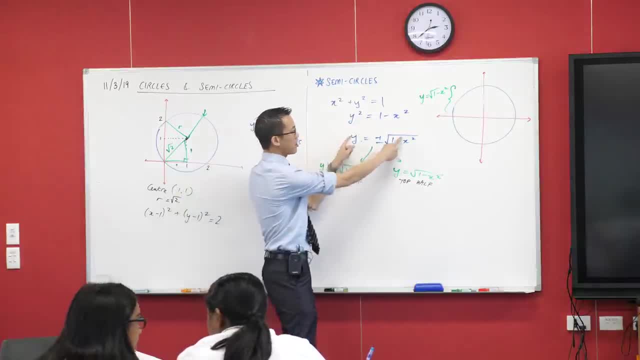 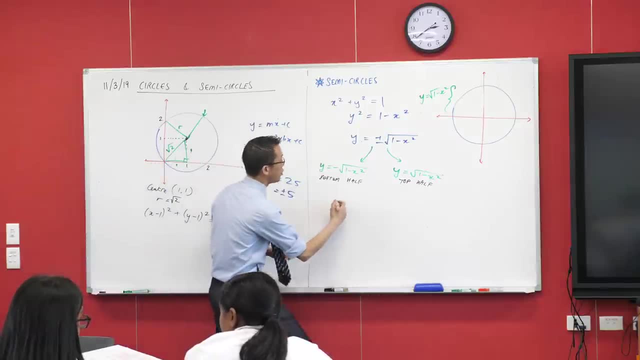 okay, Yeah, you're just like. you're literally swapping all the x's and y's around. Do you see that right? So underneath here, I don't even think you need to do the working right. You're going to get x equals. 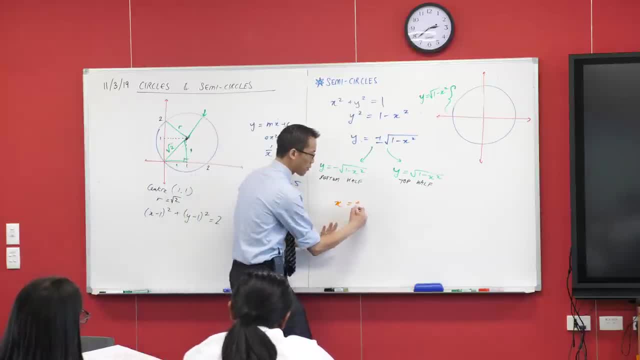 if I made x a subject instead of y the subject, you're still going to get x equals x. You're still going to get x equals x. You're still going to have a plus or minus right. You're still going to have the square root. 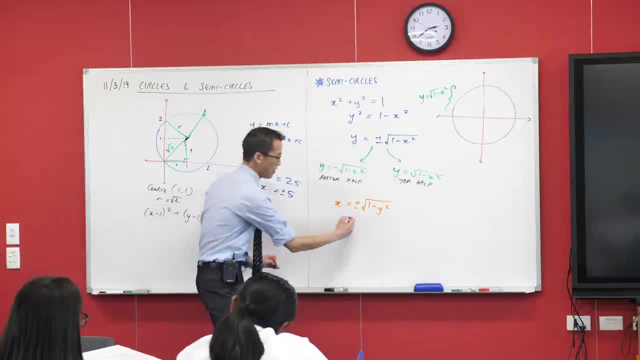 And then you're getting 1 minus y squared. Now, just like before, this is shorthand for two separate things. There's going to be the negative one and the positive one. Which one do you think is the left and which one is the right? 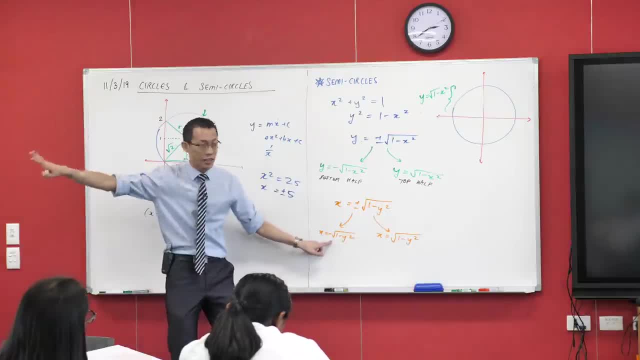 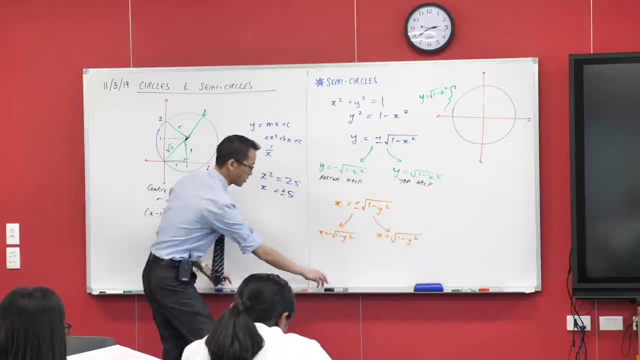 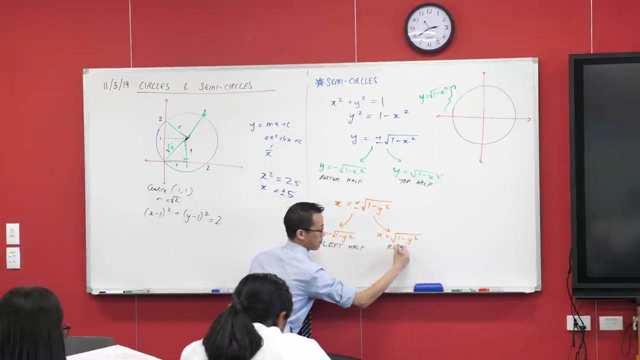 Conveniently. the negative one is to the left, because look at our axes right To the left over here is negative values of x. So this guy here is the left half And that leaves this guy as the right half And just like before, 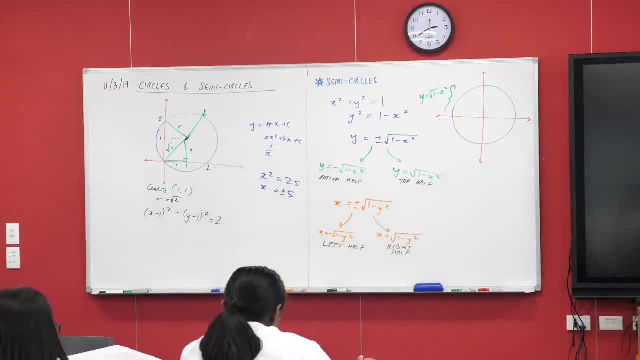 if you'll bear with me while I fiddle with my equation. I'm glad you like that. There you go. There's the right hand semicircle, just like we saw before. I made x the subject, and because x is about left and right. 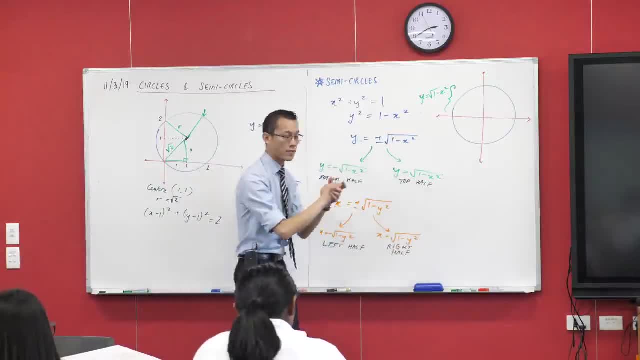 and if you're restricted to positive values, you go to the right. It's pretty neat right Now. the tricky thing is that the water gets deep pretty fast after this, and I'm going to let you guys explore this a little on your own. 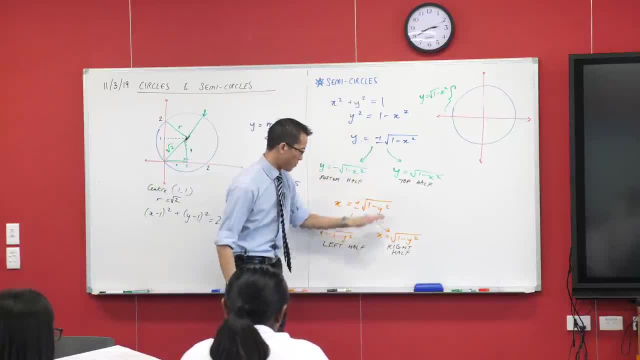 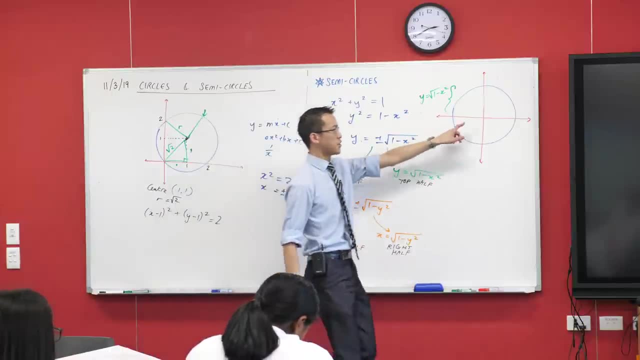 What circle were we playing with? to make the bottom on the top, the left and the right? We've been playing with the unit circle the whole time, right? So if I wanted a semicircle that was not centered on the origin, that perhaps didn't. 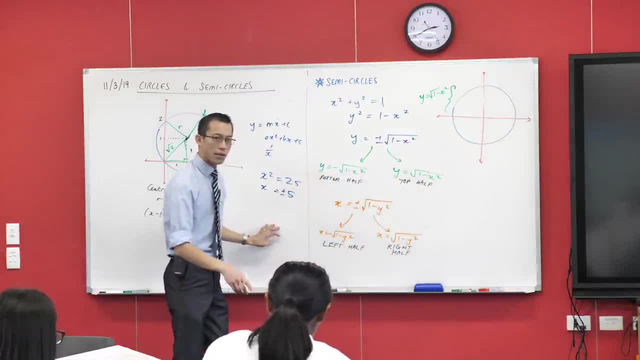 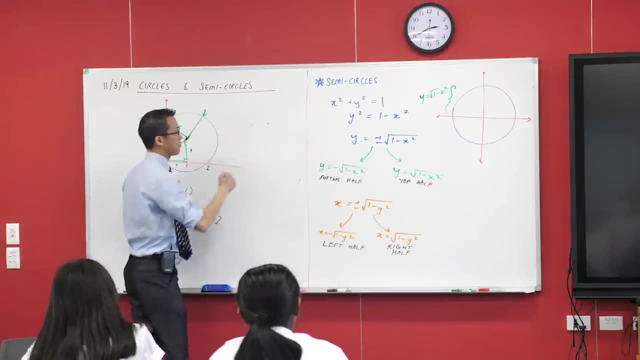 have a radius of exactly one. these numbers are going to become a little more complicated. Let me give you an example. You don't have to write this down, just think through it with me. right? What is if you saw something like 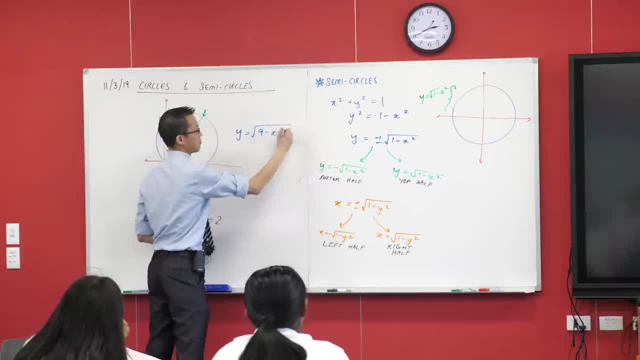 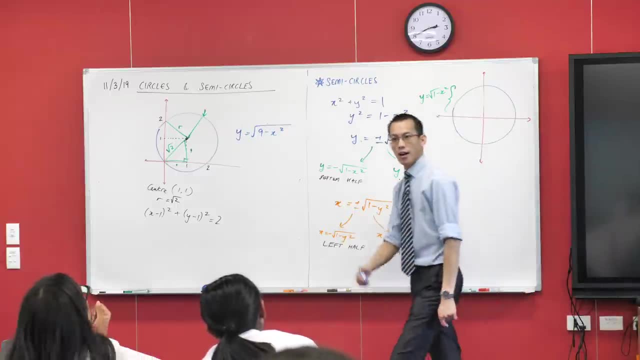 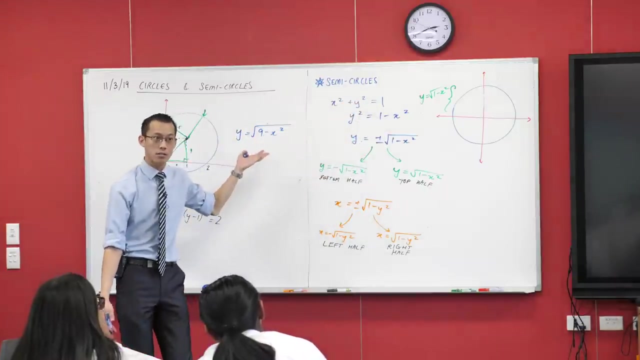 this. Okay, This is relatively simple. I've only changed one thing, Okay, so think about this. right, You could check this. You know how we started with this and then we made y the subject. right, You can do this in reverse.